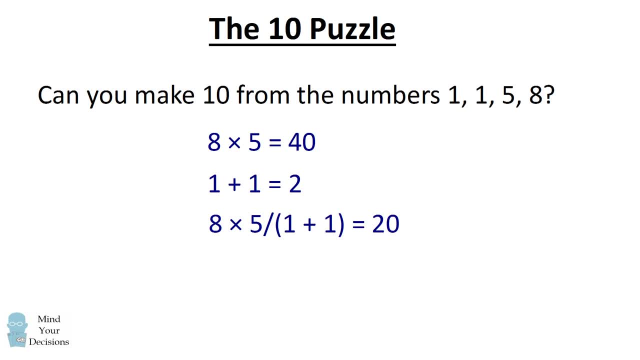 as far as 10.. So we want to reduce this by a factor of 2.. So we can try and move the terms around, Like, let's say, we move the 5 over to the denominator. If we do that, we take 8 divided by. 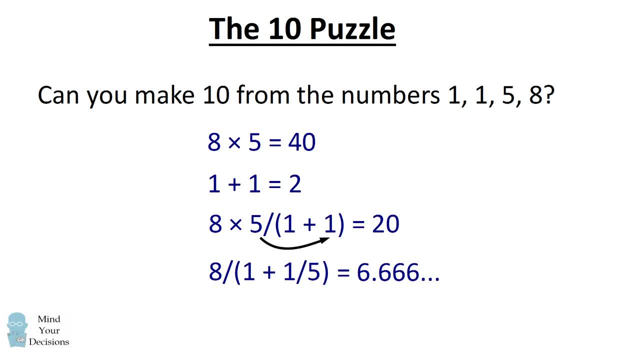 1 plus 1 fifth, and that gets us to 6 and 2 thirds. So now we're actually we've undershot. we want to get back up higher. So we could do that by reducing the denominator and changing the sign. 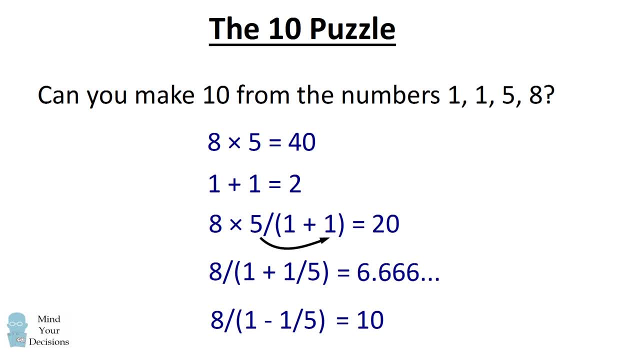 to a minus. And now, magically, we've gotten to our solution: 8 divided by 1 minus 1 fifth is equal to 10.. If you go through the steps carefully, what happens is we've grabbed one factor from the 5 and we've gotten to our solution. So now we can do that by reducing the denominator and changing. 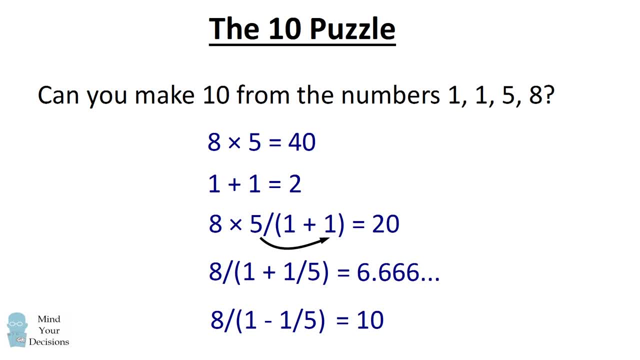 the sign to a minus. And now, magically, we've gotten to our solution: 8 divided by 1 minus 1 fifth is equal to 10.. And because the denominator is 4 fifths, we've reduced 8 by 2 factors of 2.. So we've grabbed one factor of 2 from the 8, and we've grabbed the other factor of 5 from the 5 to get us to 10.. 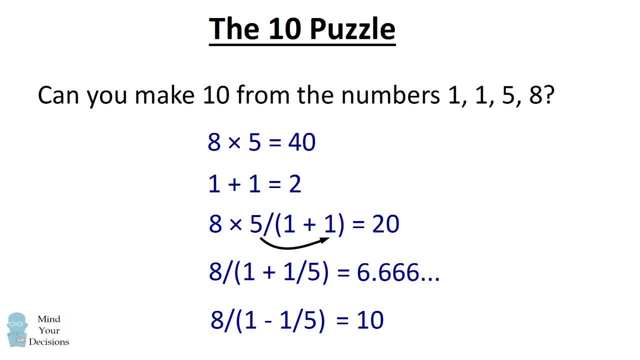 What's very interesting about this puzzle is that it's a very unexpected thing that you'd want to divide by 1 minus 1. fifth, And the other thing that's interesting is I went through and I calculated all the different ways that you could combine the numbers 1, 1,, 5, and 8 with the operations of 1, 1,, 5, and 8.. 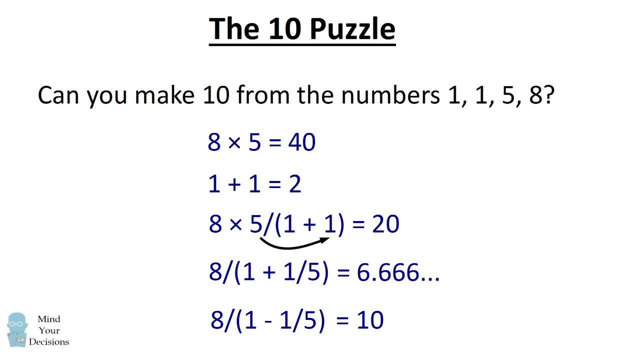 And what I found. I've linked the solution in a spreadsheet. It's got over 1,700 entries And this is the only solution. This is the only way that you can get these numbers to get to a result of 10.. 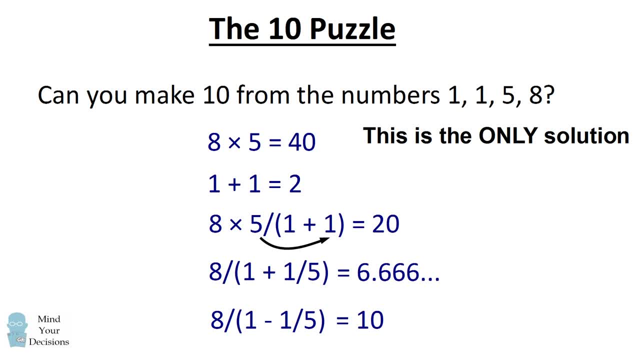 So it's a very interesting puzzle And if you look through the entries, there are really no other ways that you can arrange the numbers that have a unique solution. that's also interesting and wouldn't be hard to find out just by looking at the numbers. 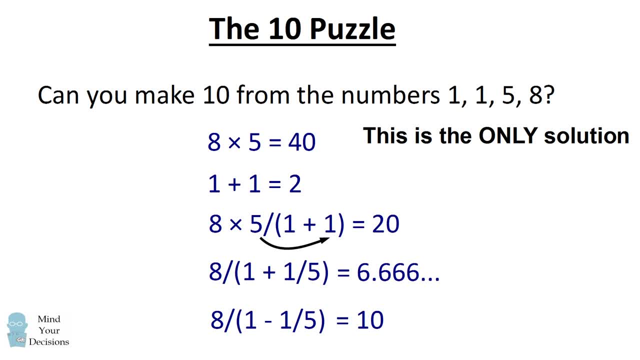 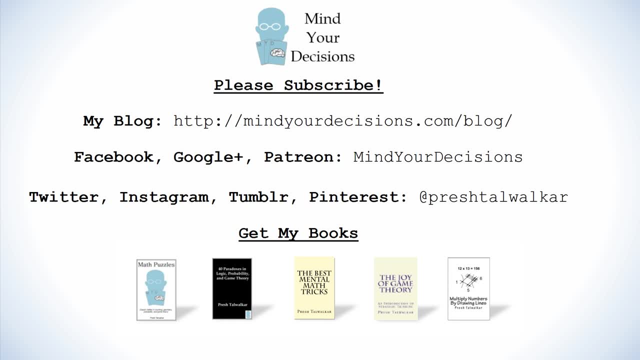 So it's a pretty cool puzzle and it's great that Google included it in a TV commercial. Thanks for watching this video. Please subscribe to my channel. I make videos on math and game theory. You can catch me on my YouTube channel And I'll see you in the next video. Bye.